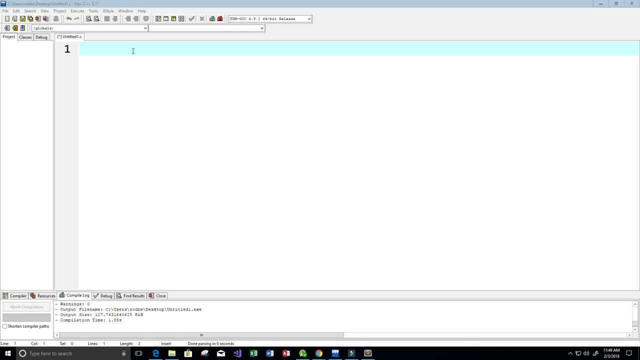 Hey guys, and welcome to this video on the C programming language. So in this video we're going to do another practice problem. We're basically going to try to find the smallest positive integer value that cannot be represented as sum of any subset of a given array, And so I'll show you guys exactly what that means. Let's go ahead and get started, for now, with a few comments. So first I'm going to give this program a title, and it's going to be exactly what I said: We want to find the smallest positive. 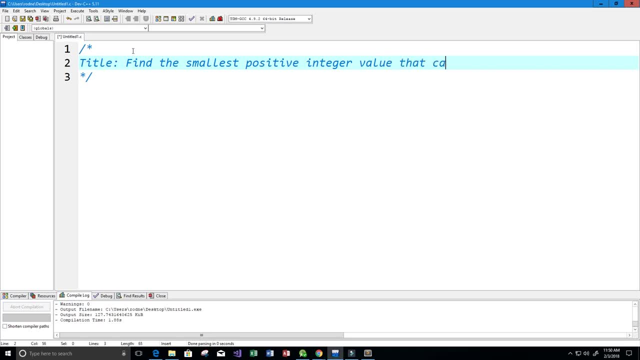 integer value that cannot be represented as a sum of any subset of a given array. All right, and I'm just going to press enter here so we can see it all on the screen at one time. Perfect. So now let me explain the problem. So, basically, we're going to be given a sorted array and the 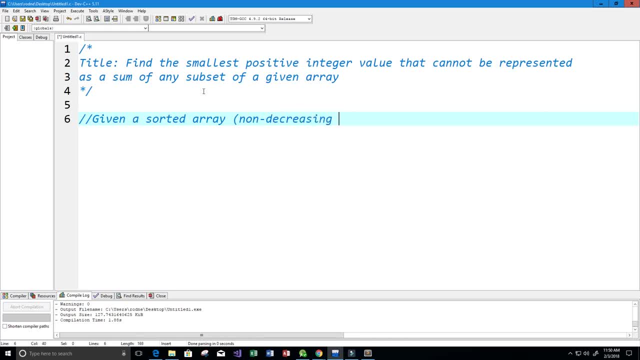 array is going to be sorted in non-decreasing order. Okay, so that means that the elements can all be the same or greater, All right, and it's going to be a sorted array of positive numbers. So, positive numbers: We want to find the smallest positive integer value that cannot be represented as a sum of the elements of any subset of a given array. 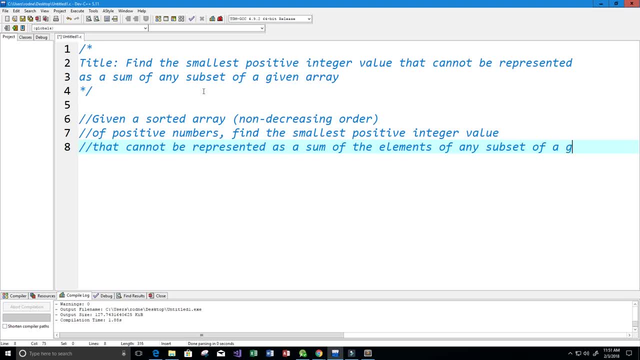 We're going to come back to that set. So it's going to be a simple trigonometric integral of positive set of a given set And we are expected to do this in big O of n times. So that basically just means- and it's not always true, but it basically means- that we're going to have to do this in 1-4 loop. 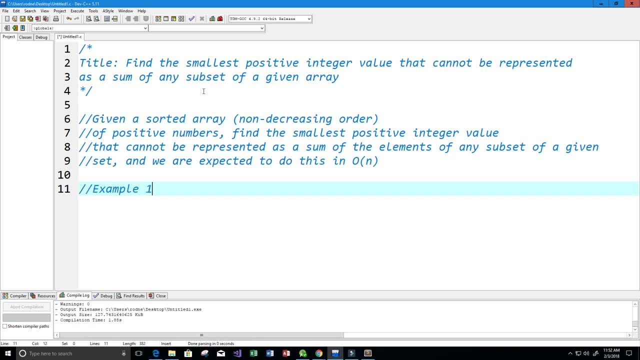 So let's give a few examples. So I say example one: here We're giving some input array. So it'd be an array and it'll have the numbers, maybe 1,, 3,, 6,, 10,, 11, and 15.. 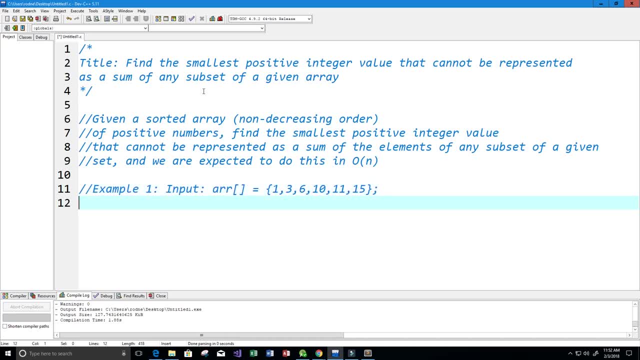 Okay, Our expected output would be the number 2, because the number 2 is the smallest positive integer value that cannot be represented as a sum of these elements in the array. Okay, So maybe I'll do an explanation here as well. Okay, So what integer values can we get from this array here by summing up the numbers? 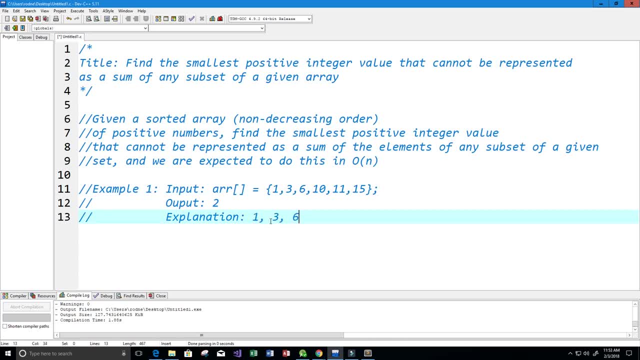 So we could get 1,, we can get 3,, we can get 6,, we can get 10,, we can get 11,, we can get 15.. Okay, Well, that's obvious, because they're all there. But now, what subsets can we get by adding these numbers together? 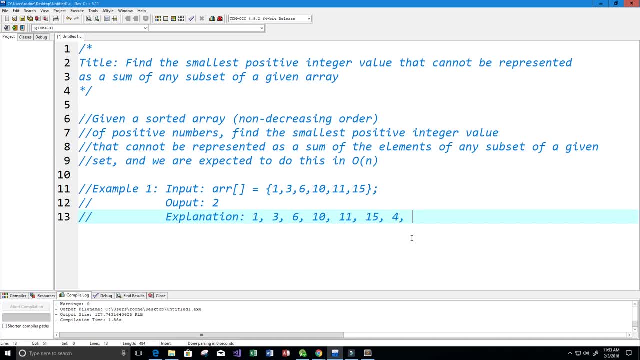 So we could get 1 plus 3,, which is 4.. Okay, Okay, We can get 1 plus 3 plus 6,, which is 10.. We already have a 10, so I don't need to write it again. 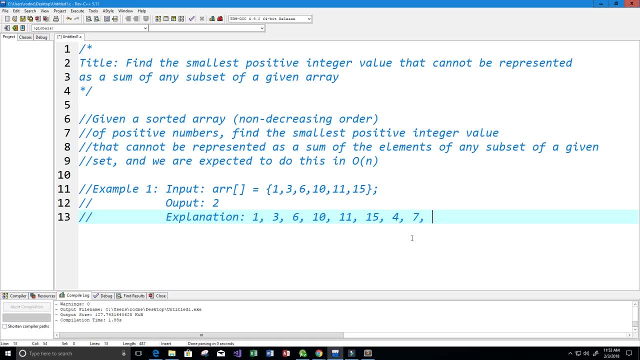 We can get 1 plus 6,, which is 7.. We can get 10 plus 11 plus 15,, which is 36.. And we can get 1 plus 3 plus 6 plus 10,, which is 20.. 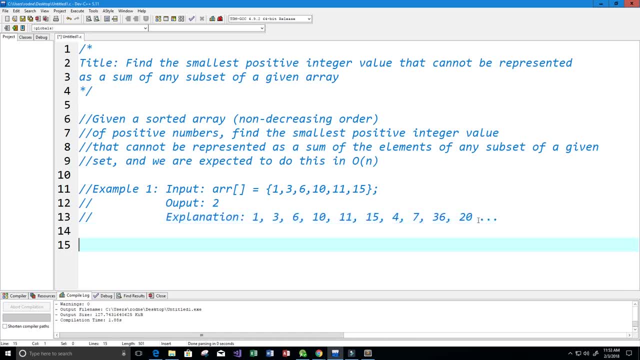 And so on and so forth. Okay, So let's give another example. Make sure that, Make sure that we are understanding the problem that we want to solve. So we're going to input an array, something like 1111.. Now this array is still sorted in non-decreasing order. 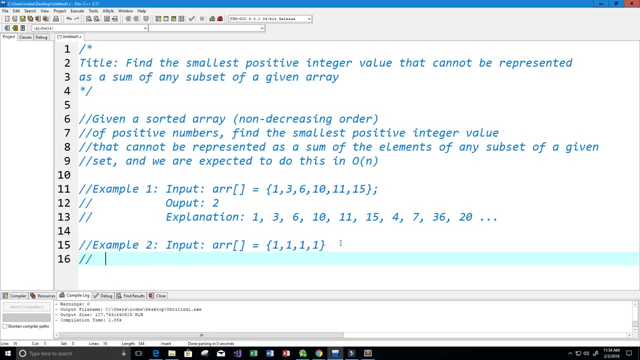 All the values are the same, All right, So what would our output be? Well, our output here would be the number 6.. No, the number 1,, 2,, 3,, 4. It would be the number 5.. 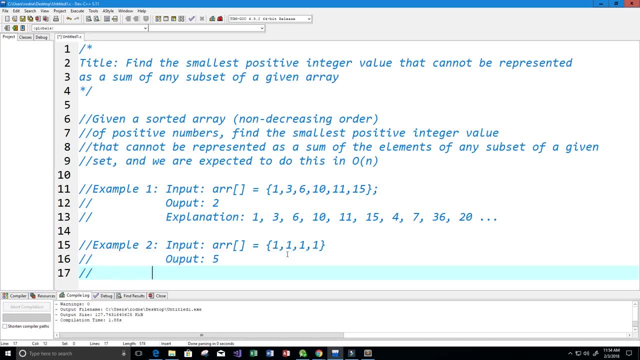 All right. And why is that? Why is it 5?? Let's see here Explanation. So we can add: Well, we get 1.. We can have any of these elements as 1.. We can get 2. We can get 2 by adding any 2 of them together. 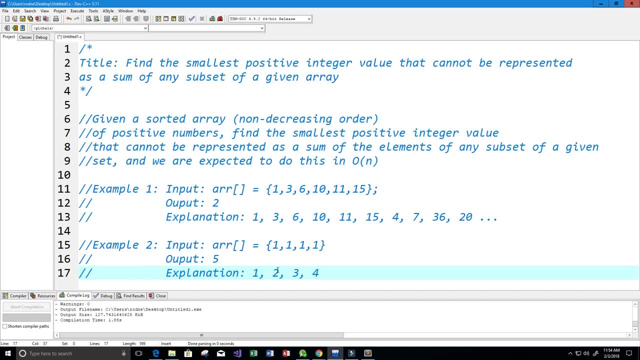 We can get 3 by adding any 3 of them together, And we can get 4 by adding any 4 of them together, or all 4 of them together. Now, the next smallest positive integer value that cannot be represented using this set would be the number 5.. 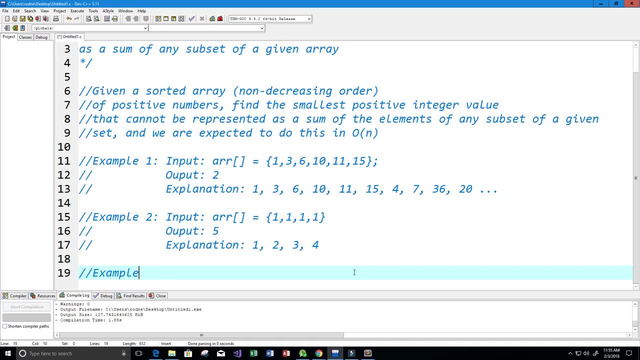 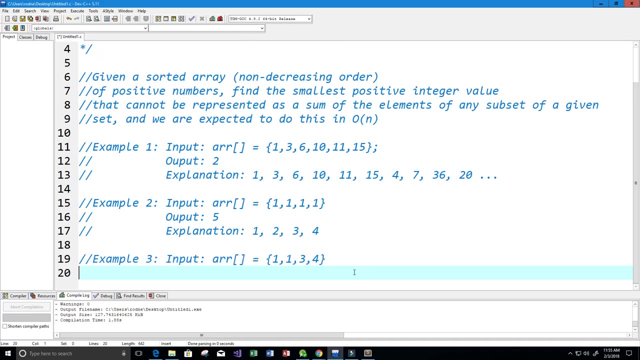 All right, Maybe another example, And I'll probably do one more after this one. So let's see, We get our input array and it's something like 1, 1, 3, 4.. And I keep misspelling output up here, apparently. 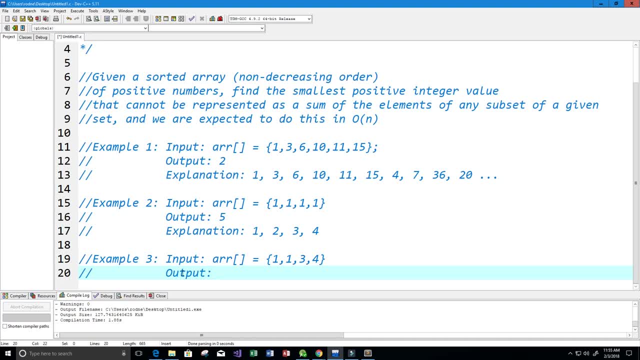 Okay, So output What's the smallest integer value that cannot be represented by this array, And that would be the number 2.. 2,, 5,, 9,, 2,, 3,, 4,, 5,, 6.. 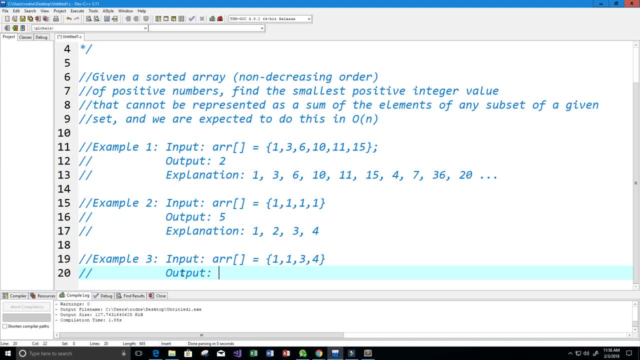 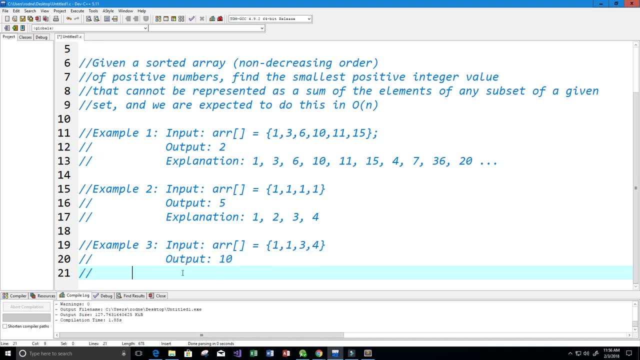 We can get 6,, we can get 7,, we can get 8,. yeah, we can get 9.. So the smallest integer value is 10.. And right now, what I'm basically doing is going through all the possible combinations, or you know. 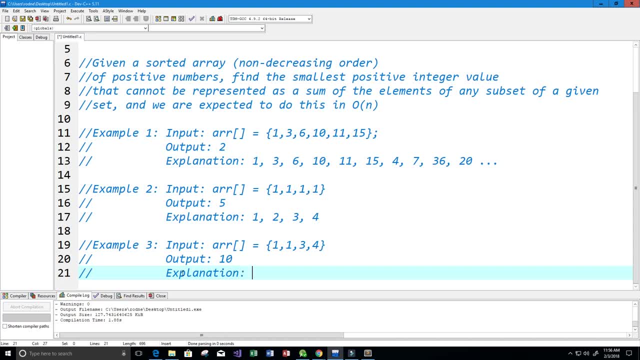 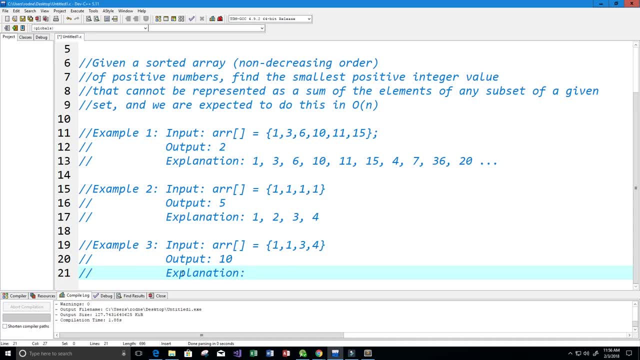 This array can create, And we can do that in two for loops, but we can't do that in one for loop, Not that way, Okay. So explanation here: we can get 1 from the 1.. We can get 2 by adding the 1 and the 2.. 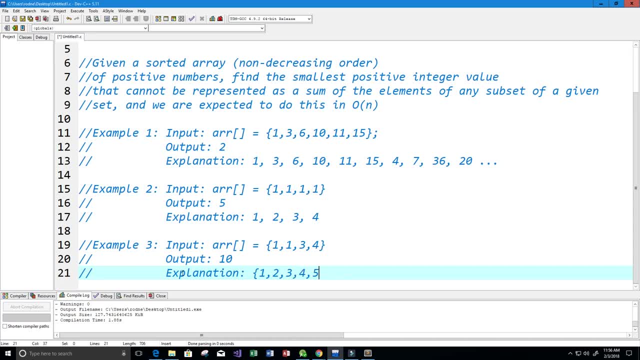 We can get 3 from the 3.. We can get 4 from the 4.. We can get 5 from adding the 1 and the 4.. We can get 6 by adding both of the 1s and the 2, I'm sorry, both of the 1s and the 4.. 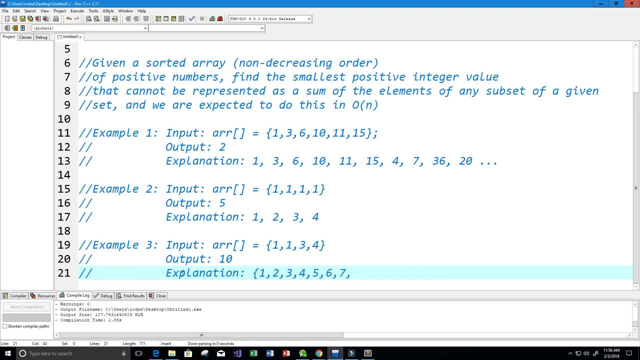 We can get 7 by adding the 3 and the 4.. We can get 8 by adding a 1,, a 3, and a 4.. We can get 9 by adding every single element in the array, but we cannot get the integer. 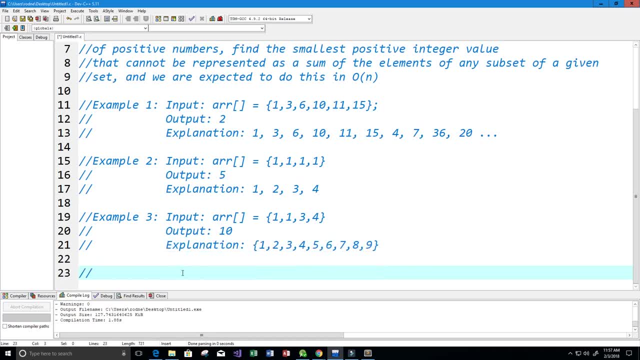 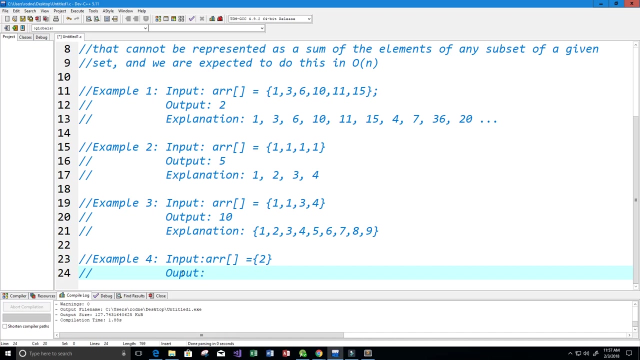 value 10 from this array. Okay And last but not least, this is an important example, And we're basically given an array like this, So all it contains is the element 2.. Okay, And what is our expected output? You may think that it's actually 2, but no. 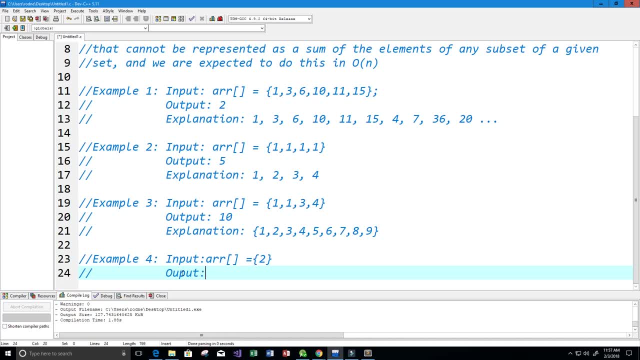 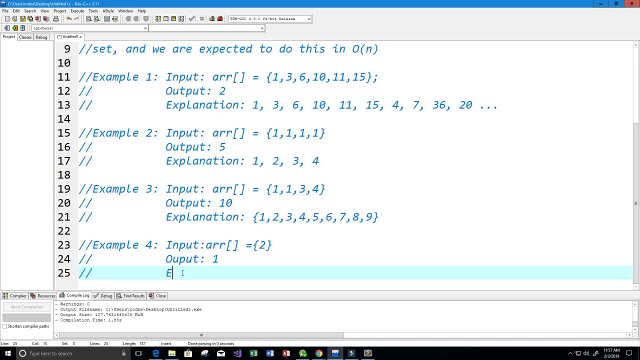 The smallest possible integer value that cannot be represented by this array is the number 1.. All right, And I can explain this, but I don't think it really needs an explanation. The smallest positive integer value is 1.. All right, So let's go ahead and get started on this problem. now get coding. 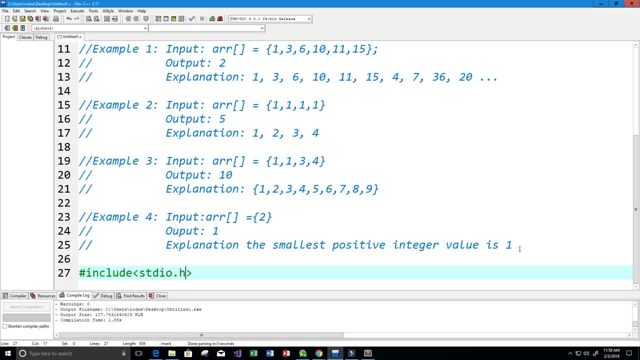 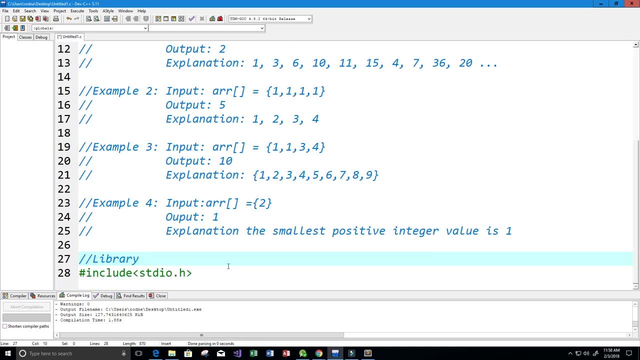 So let's set up our. let's set up our main, our main function and our library and the syntax, All right. So right now I'm just creating our library, or not creating. I'm including our library. Now I'm creating our main function. 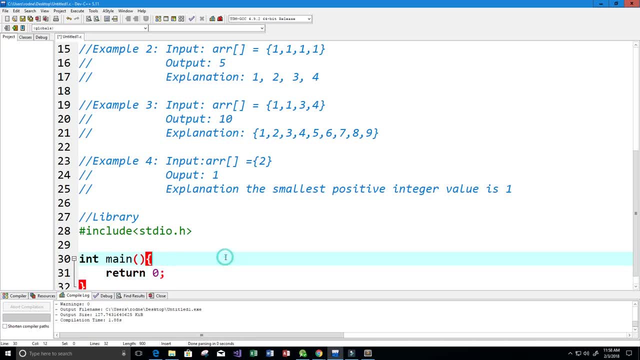 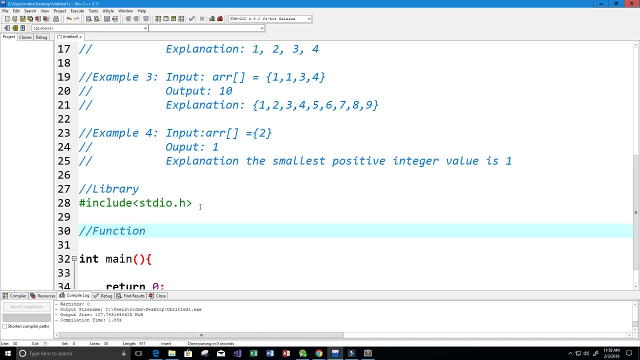 Okay, And return some integer value. I'm going to return 0.. And this is just setting up our program. So now I want a function that's going to return the smallest positive integer value And it needs to return an integer. So it's going to return an int and I'm going to call it small int. 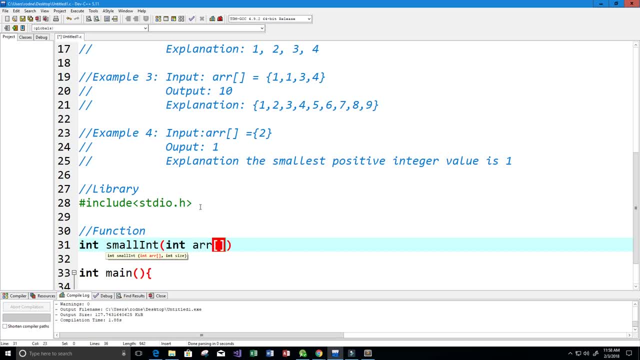 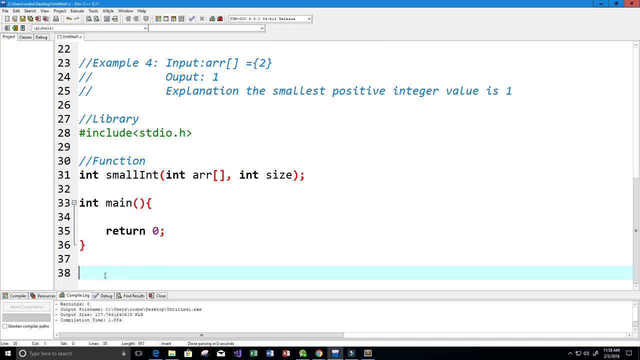 And now small int needs to take in an array And we need to know the size of that array. Okay, So I'm going to take in the array and the size of the array. All right, Now I'm just going to copy this here: 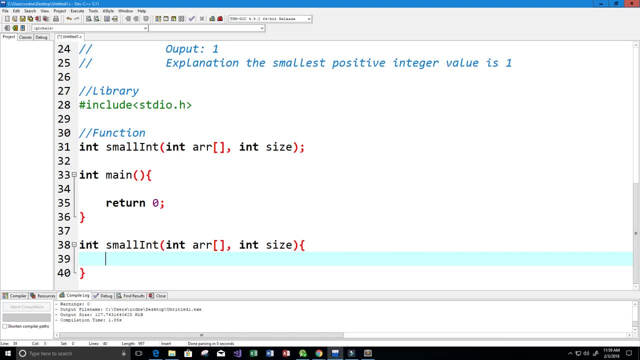 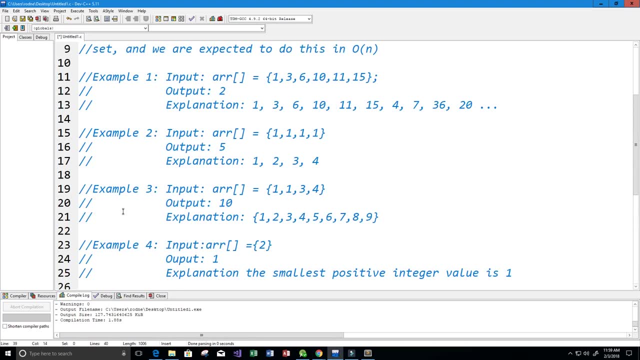 And this is where we're going to actually work on our function, And because right now it requires that I return an integer value, I'm just going to return the value 0.. And I'm going to run our program to see if everything's syntactically correct and see. 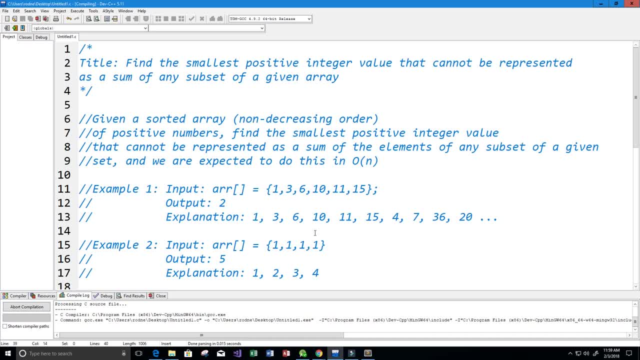 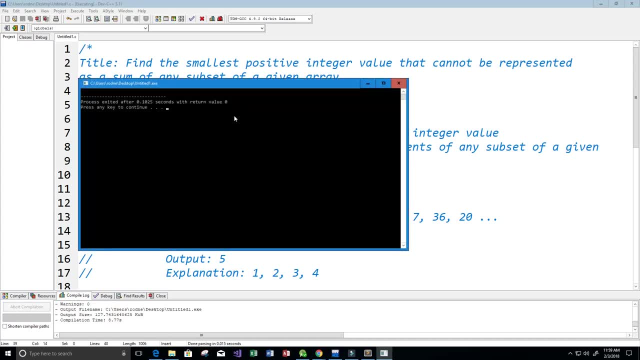 if it compiles, All right, All right, So let's give it some time here. All right, It looks like it's doing something and, yes, we're here. So it looked like it compiled with no errors, which is nice. 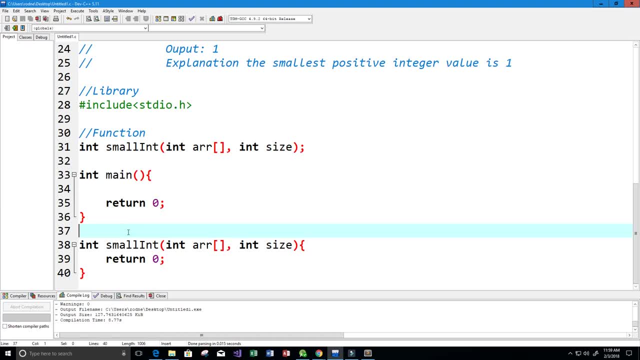 All right. So now we have to start thinking about how to code this. So we're going to be given again some integer array. I'm going to call it R, And it'll have values like 1,, 3,, 6,, 10,, 11,, 12,, 13,, 14,, 15,, 16,, 17,. 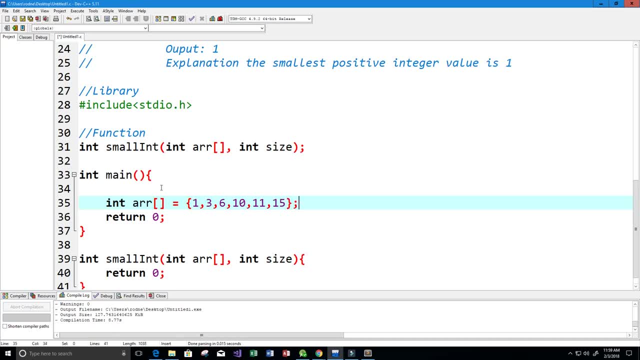 18.. All right, And then we need to know the size of the array. So I'm just going to create an integer variable called size, And the size of the above array is 6.. We have 6 elements: 1,, 2,, 3,, 4,, 5, 6.. 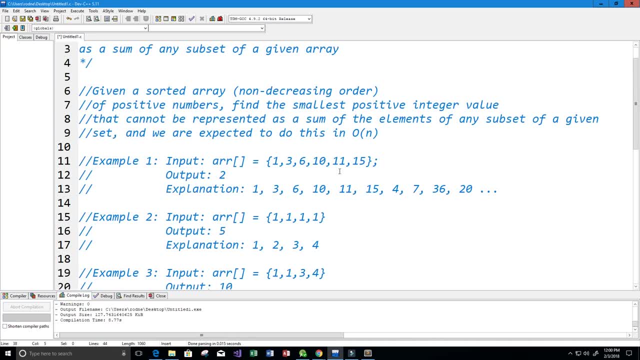 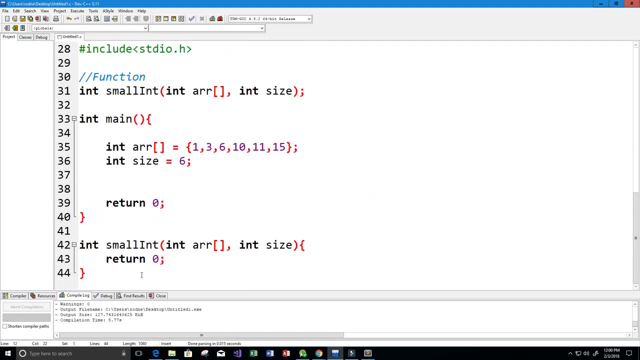 OK, And of course this is from our example up here. So the expected output is 2.. All right, So let's go to our well, let's actually let's create another variable And let's just call it output, maybe. 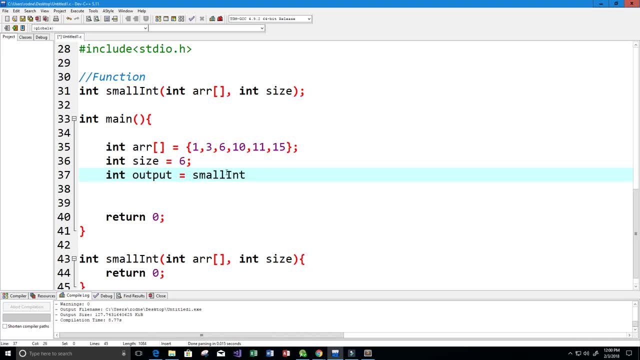 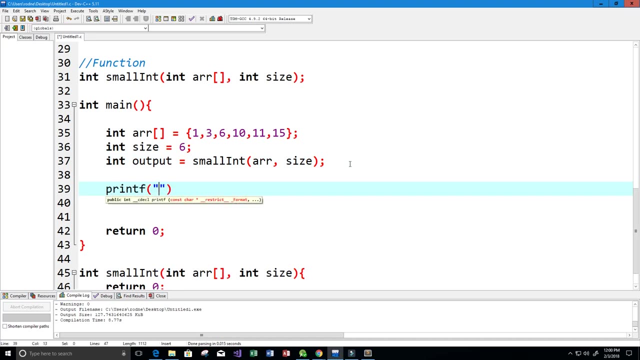 And output will be equal to our function- small int- And it's going to take in the array and it's going to take in the size, OK, And that's going to be our output, And then we're going to print this to our console. 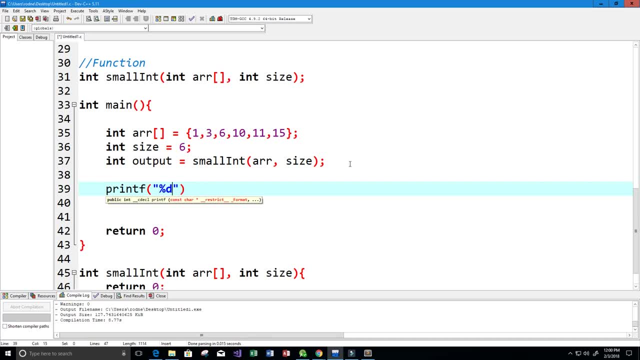 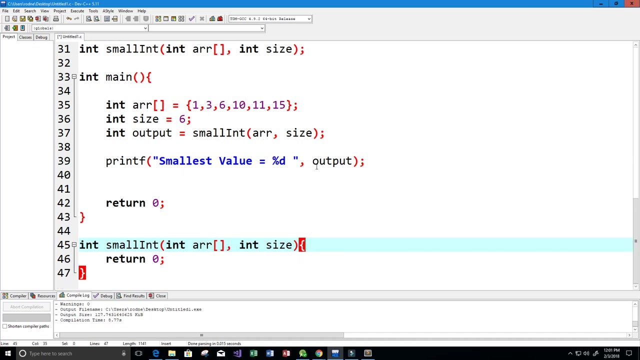 So I'm going to say %d, and then we're going to use output here And then that should give us our smallest value. so maybe I'll say smallest value equals %d. OK, So of course %d. we're getting that from our variable output. 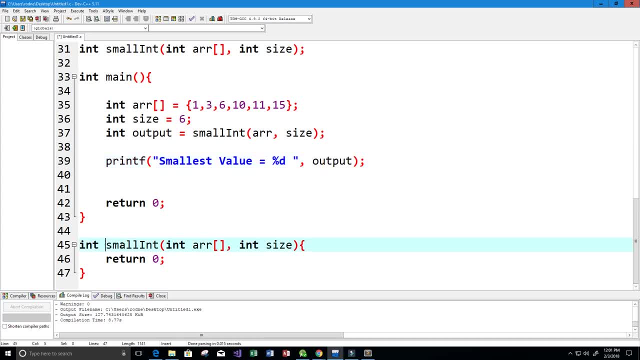 OK, And, as a matter of fact, let's go ahead and run this right now: Small int: the function is going to return 0.. So all this is going to return 0.. So our output is going to be equal to 0.. 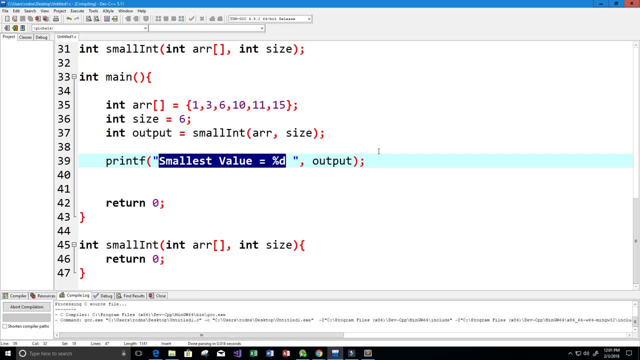 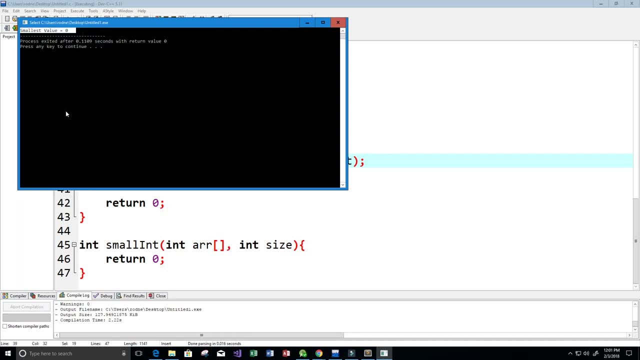 So the smallest value equals 0. So let's run this and see if we get 0. And we do up here. It says smallest value equals 0. It may be hard for you guys to see, depending on how you have your screens and what type. 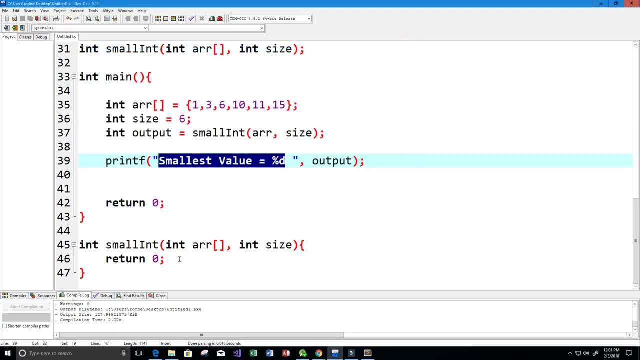 of screens you have. But it basically says smallest value equals 0,, as expected. Now, of course, the smallest positive value cannot be 0. It's going to be 1.. So let's start creating our function just like that. 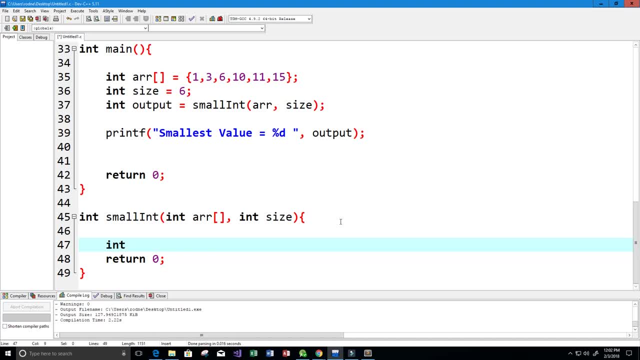 So I'm going to call the smallest value, the sum, OK, And the sum is going to be 1.. So this is going to be the smallest value that we can return. So I'm going to return sum in our function here. Let's run it. 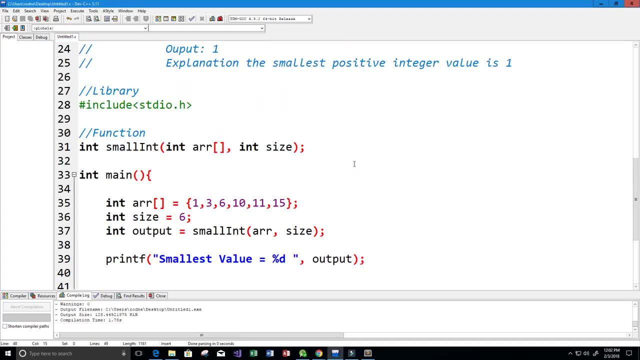 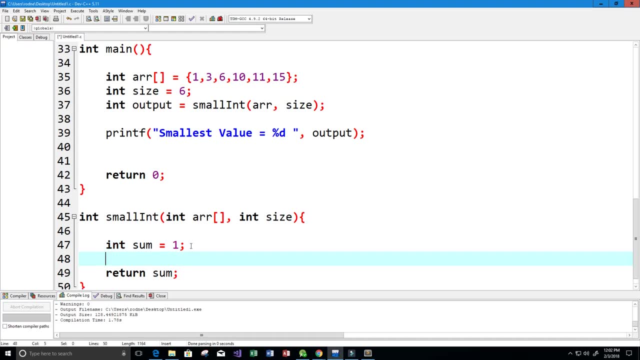 And right now? Yes, Smallest value equals 1.. So that's still not the answer that we want. We want the answer to be 2.. We want the output to be 2.. All right, But we know that the smallest integer value, or possible integer value, is 1.. 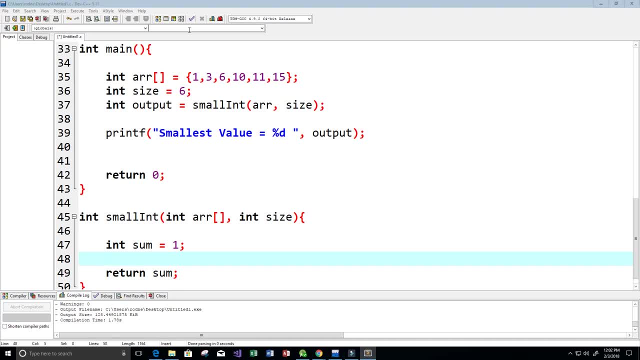 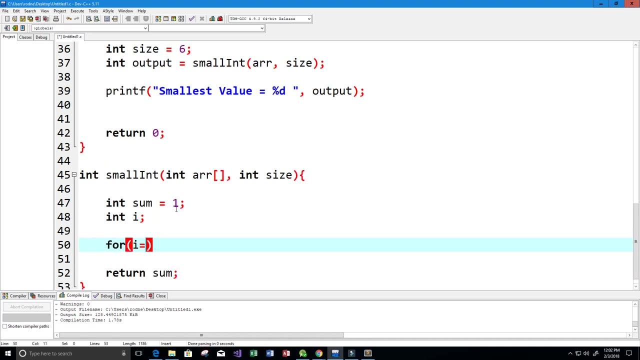 Now, I also said that we want to do this in a for loop, Right? So we're going to need a variable to loop through. So I'm going to create our variable, i, And let's go ahead and create our for loop. We need i to run from 0 because we're going to use i as an index for our array. 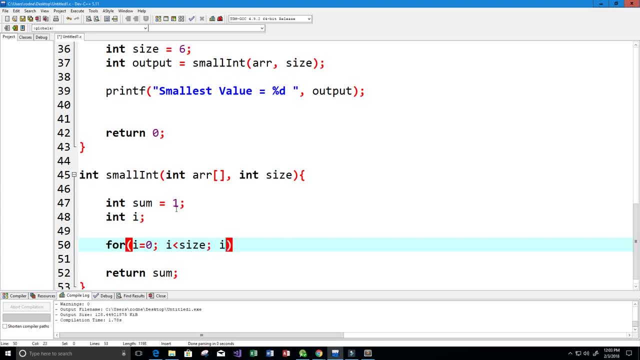 So i is going to be less than the size of the array And then i is going to increment by 1 each time. All right, And now, within this array, the reason why I chose sum is because we're basically going to have to sum up the elements in the array. 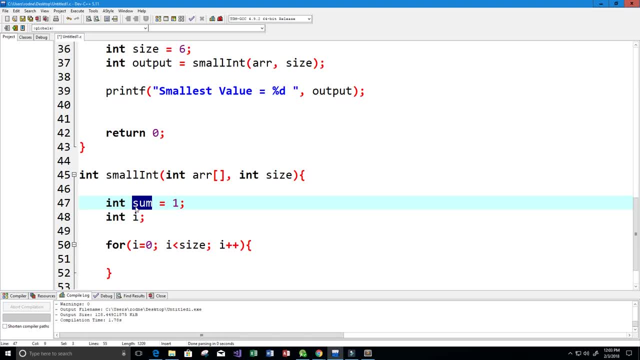 And kind of compare them to the next element to see if it's, to see if sum is greater than or equal to that next element. OK, So that was a lot, But now all we're going to need is an if statement here. 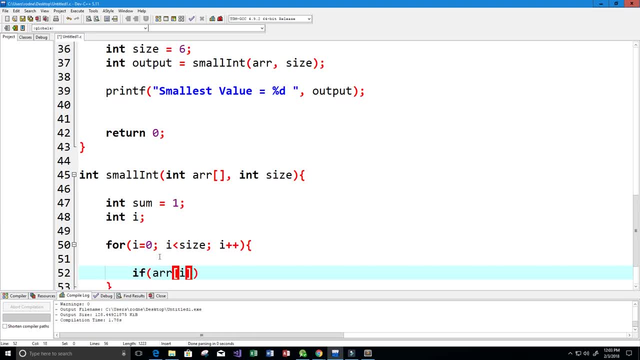 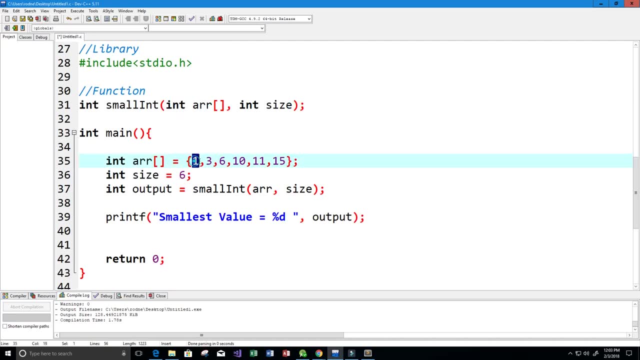 We're going to check to see if the element at position i- so that could be element at position 0,, 1,, 2,, 3,, 4, 5.. So it could be the element 1, the element 3, the element 6.. 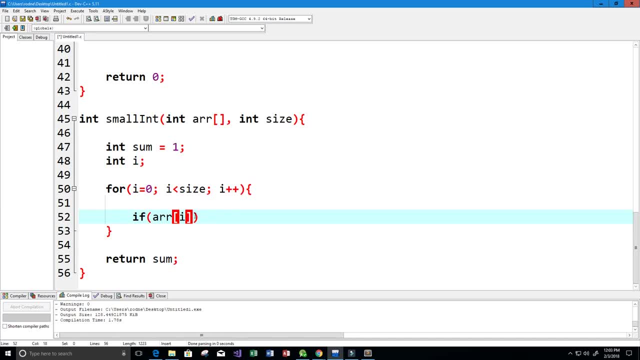 All depends on whatever the value i is. So we're going to loop through all of those elements And we're going to check to see if that element is less than or equal to the sum. All right, If it is less than or equal to the sum, then we can, we can add that element to our sum. 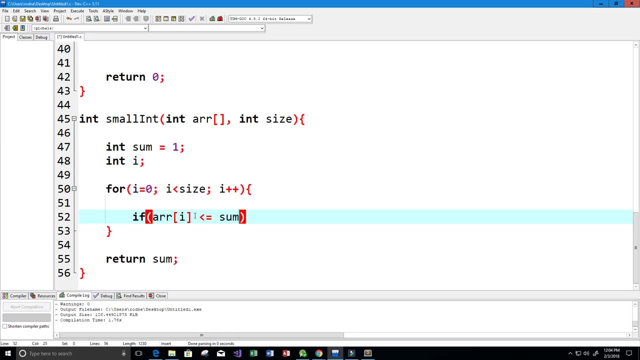 And if it's not, Then Then every other element behind it will not be less than or equal to sum as well, So sum will never increase. OK, So if the array at position i is less than or equal to sum, then we can add to sum. 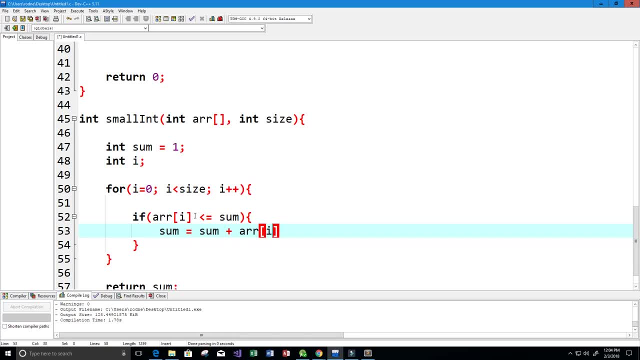 So sum is going to equal sum plus the array at that, I'm sorry- the element, The element at array position i. And again, if, if this element, if this element is greater than sum, then we won't be adding any more of the elements to our sum. 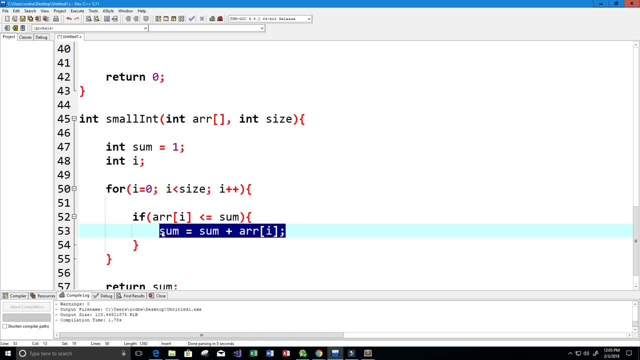 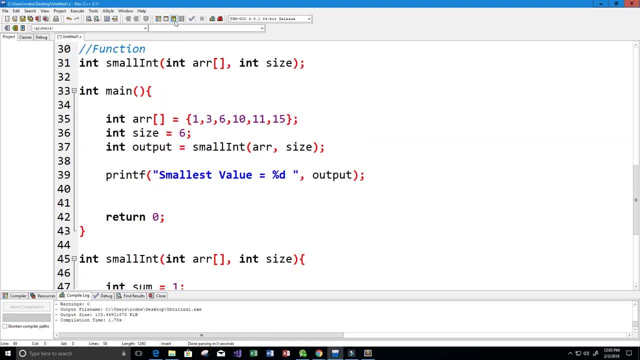 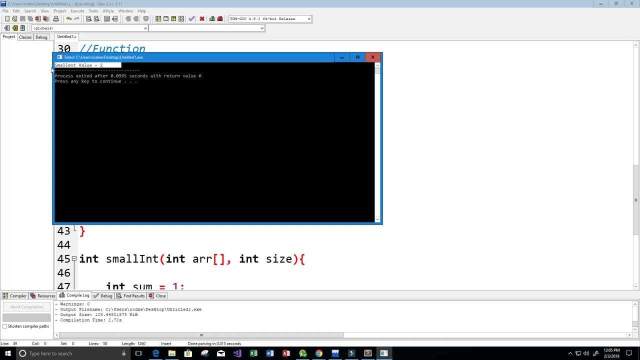 OK, We can just stop there. We're done. And we found the smallest positive integer value- All right, And so let's go ahead and give this a run, All right? So now we see that we get the smallest value equals two. 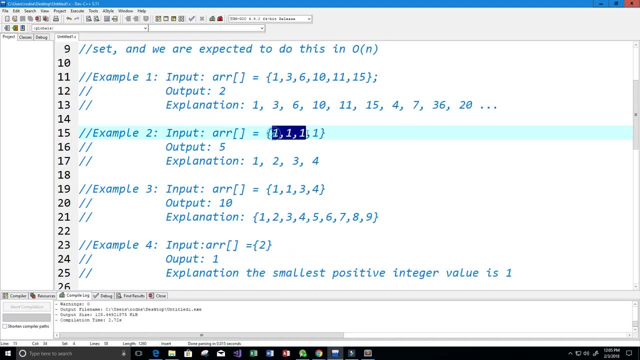 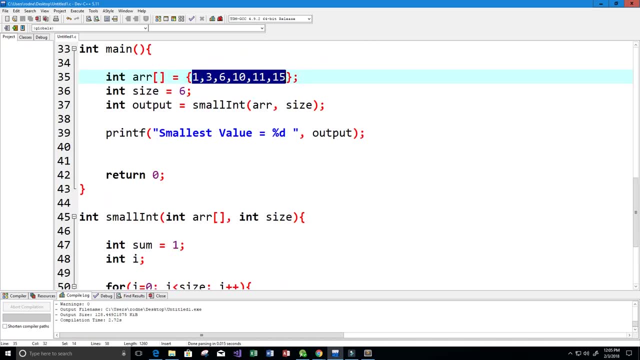 So let's copy this array here and let's see if we get the output. five, like we expect. So I'm going to put all those elements there, and now the size has changed to four. Maybe I should make this more dynamic, but let's go ahead and run this. 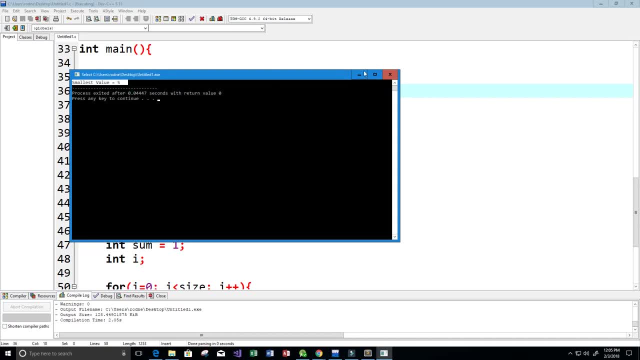 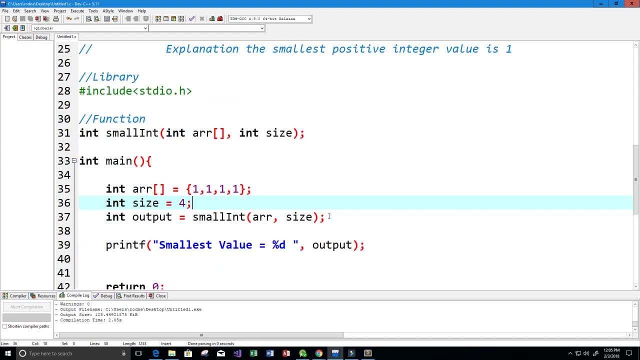 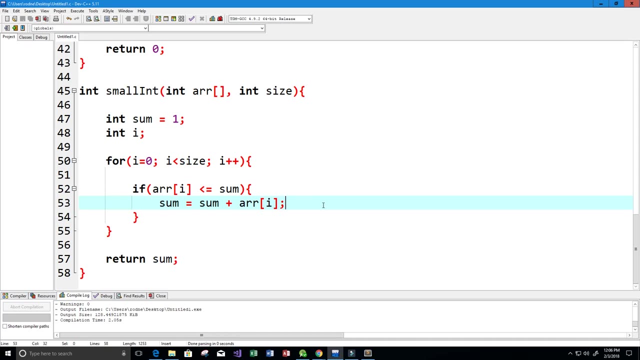 And so now we get the smallest value equals five, which is exactly what we expected from our output. So this is one solution to this problem. I have another solution as well that I might put up here, And hopefully you guys understood the problem and hopefully understood how I solved it.